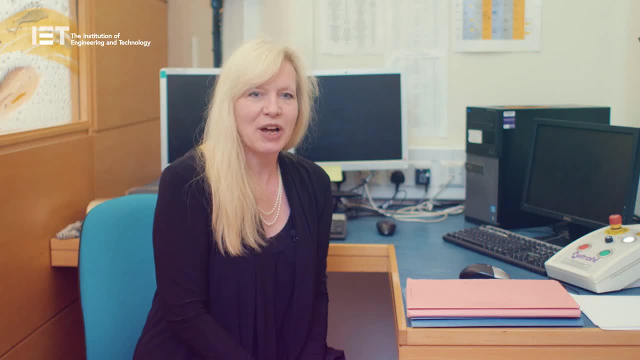 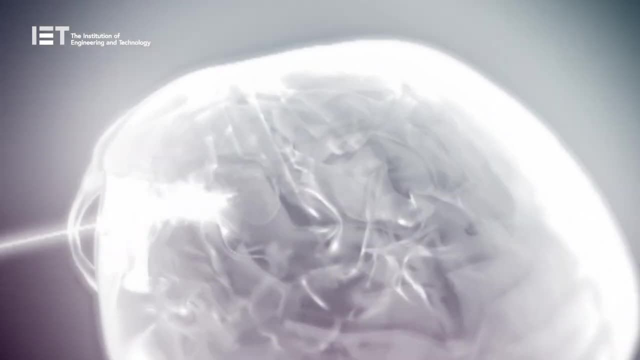 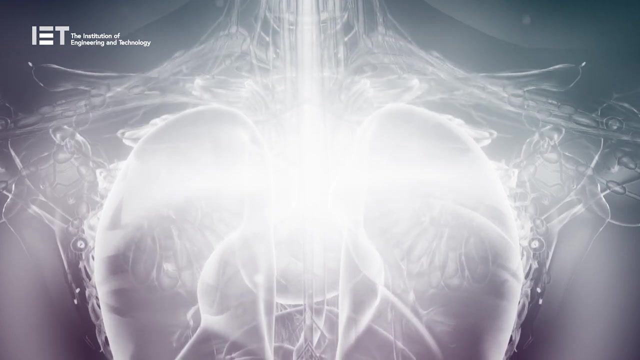 We now try and conform the dose to the tumour. So, if you imagine this, we shape the radiation dose around the tumour so that we can actually put in as much damage to the tumour and as little damage to the healthy tissue, which enables us to give patients a treatment that gives them fewer side. 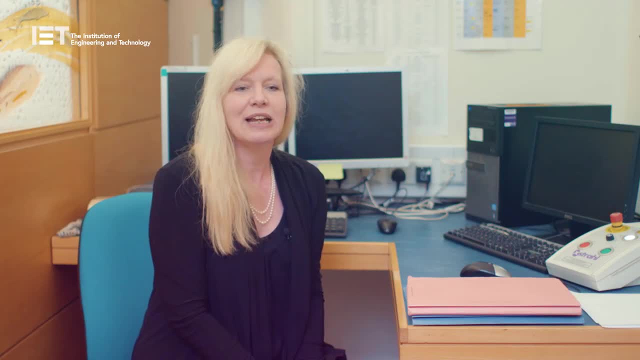 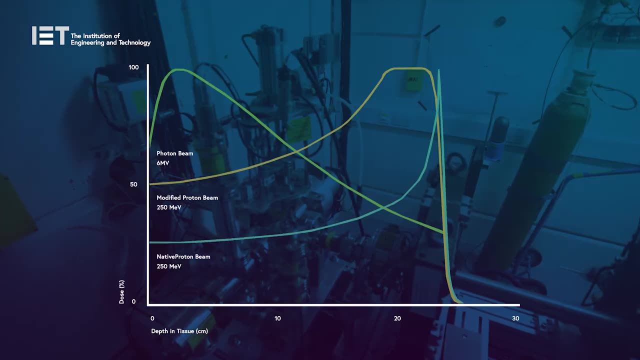 effects and better outcomes. Radiotherapy delivers radiation to the tumour in a number of different ways. Protons deposit their dose in what's called a brag peak and we can change the energy, so we have what's called a spread-out brag peak, But it's the way in. which the energy is deposited. This can either be done by x-rays, protons or brachytherapy. In the UK, 40% of patients who will be treated are children, and that's because one of the advantages of protons is that they put less dose into the healthy tissue Because of the sharp distal end. 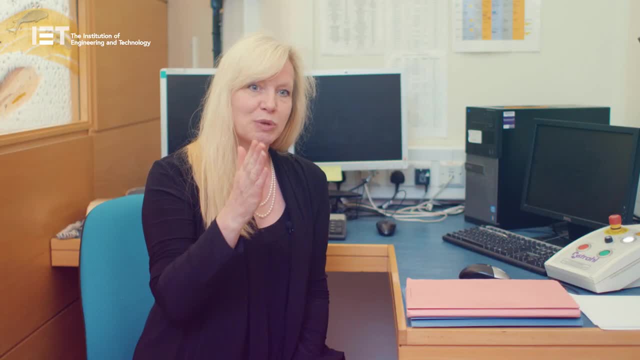 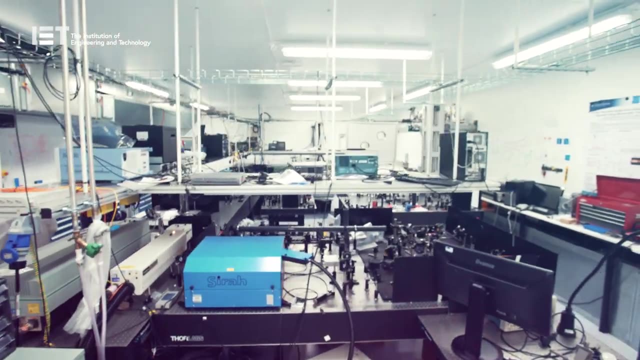 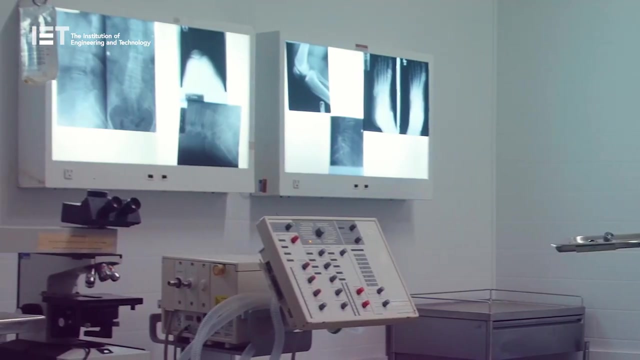 of the brag peak. you don't have any toxic dose, which means it's great for treating tumours that are close to a critical organ. However, this is not the only area of research. Particle accelerators also generate x-rays, a medical electromagnetic imaging system that creates pictures of the inside of your body. 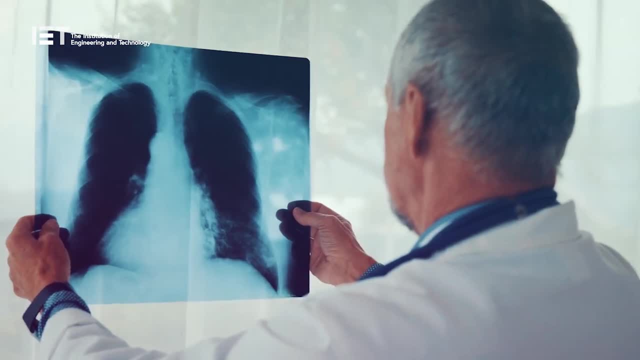 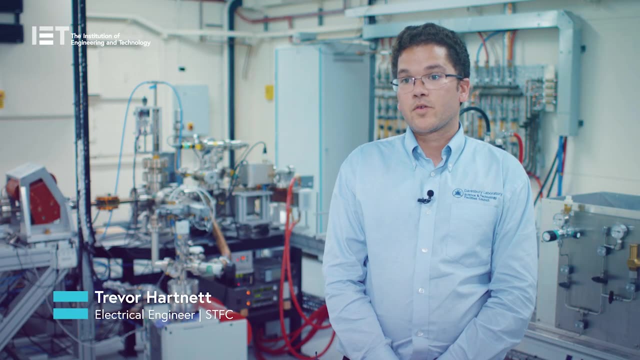 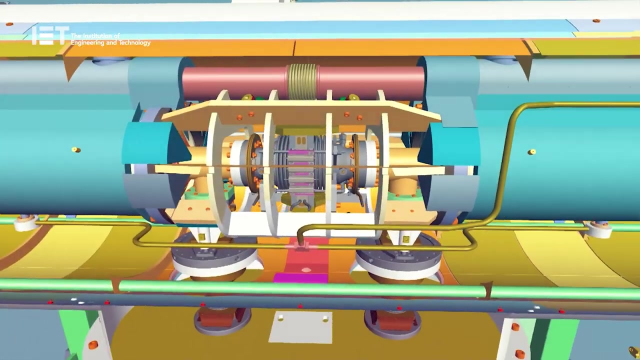 The most common use of x-rays is checking for broken bones, but they can also spot pneumonia or even certain types of cancer. Our linear accelerator is comprised of three main parts: an electron gun to produce the electrons, an accelerating cavity and a microwave RF source to produce the microwaves for acceleration. 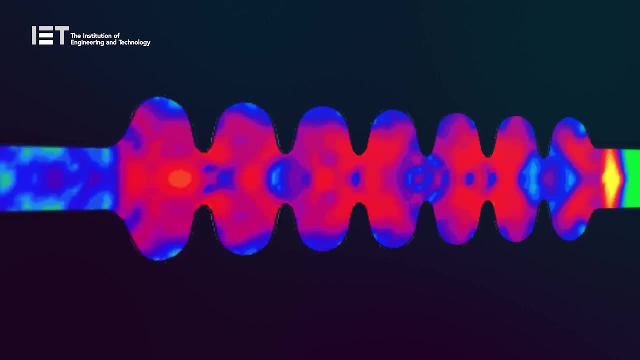 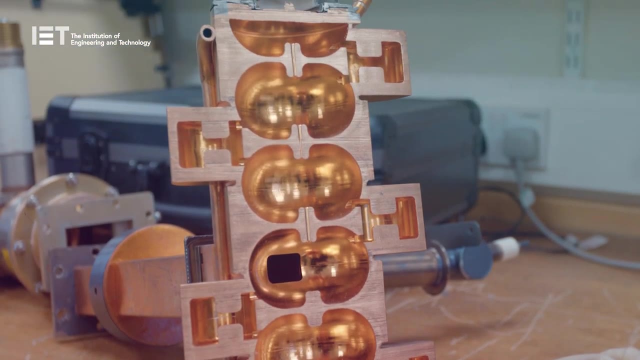 The electron beam interacts with the microwaves to accelerate along the cavity, and then it can be bent by a dipole to create an x-ray source. X-rays create electrons. by a process called bremsstrahlung, Electrons are accelerated. 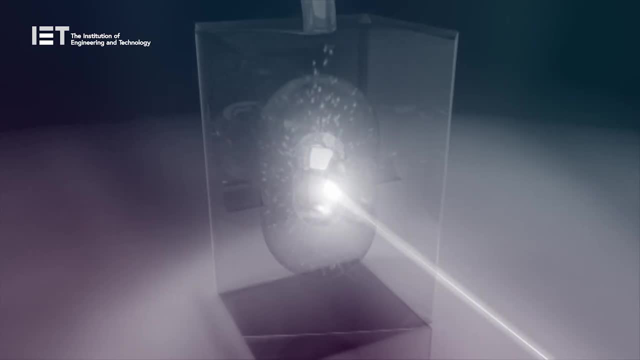 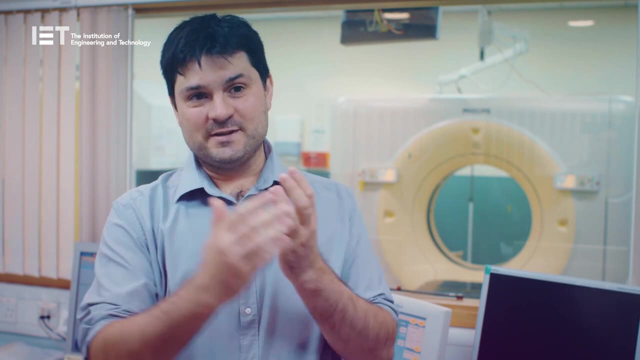 so almost light speed, 0.96 Cs, into a very, very dense metal. It's more like tungsten. The electrons interact with the atoms at the centre of that and the nucleus decelerates the electrons and this deceleration loses energy and that has bremsstrahlung radiation. So that's the process. 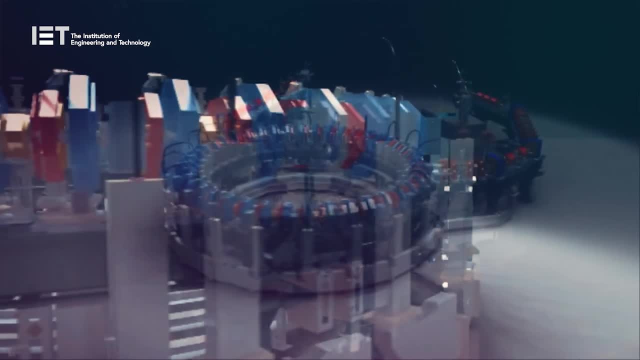 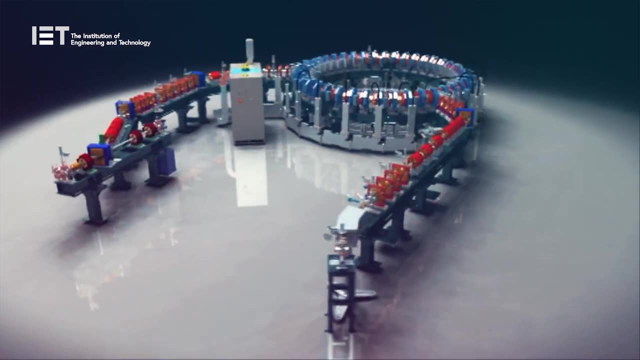 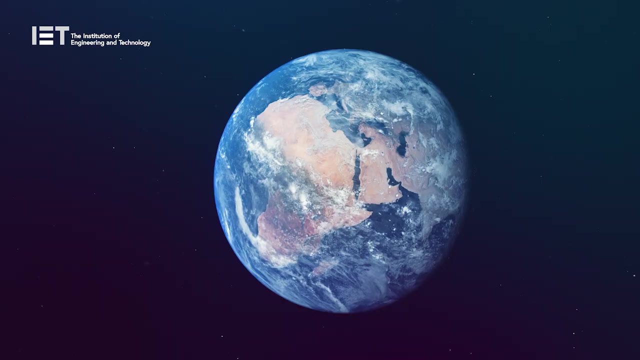 that's used. Particle accelerators are an incredible invention, One of the 21st century's most exciting frontiers of science. accelerator science has secured a key spot in a science against cancer, the search for cleaner, greener energy options and our understanding of. the universe.